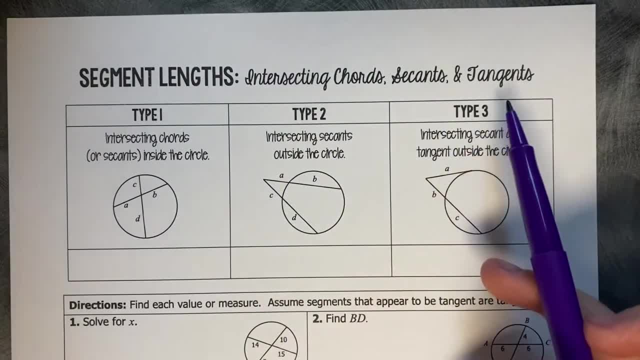 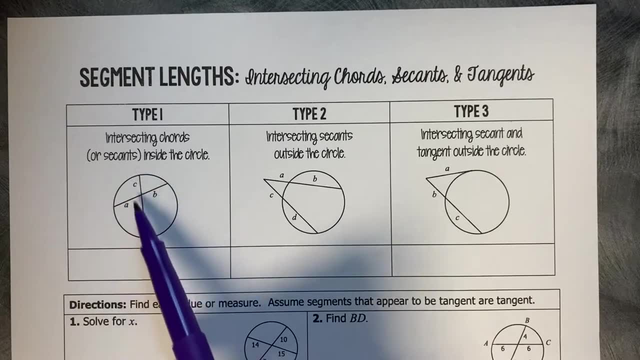 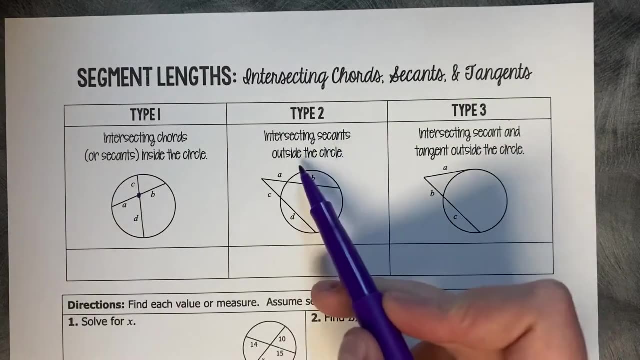 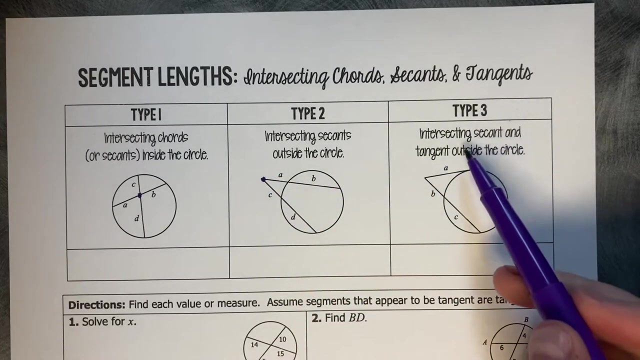 Segment links Intersecting chords, secants and tangents. Type 1. Intersecting chords inside the circle, So the intersection lands within the circle. Type 2. Intersecting secants outside the circle, So an exterior to secants. And type 3 is an intersecting secant and tangent outside the 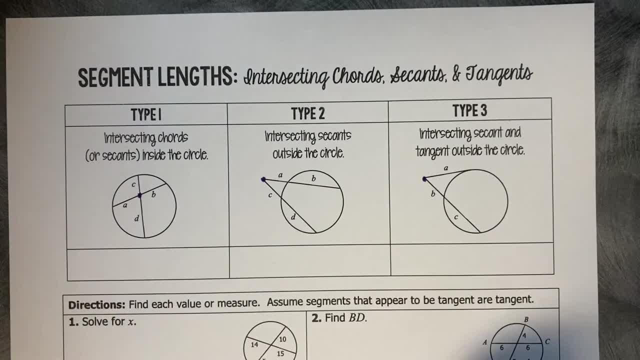 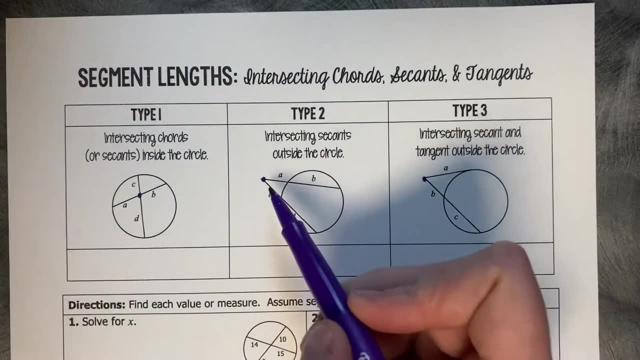 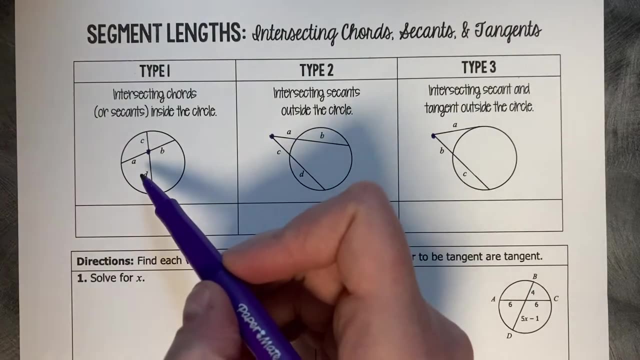 circle. So one length is a tangent and one length is a secant. So we're asking about lengths of lines, not angles of our connecting segments. So we did angle work in the last couple of sections and now we actually want to know how long each of these lines are. 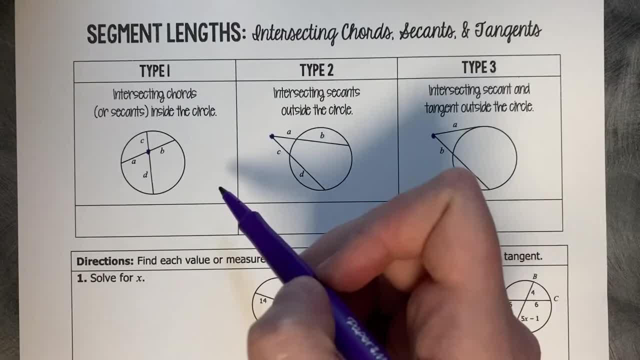 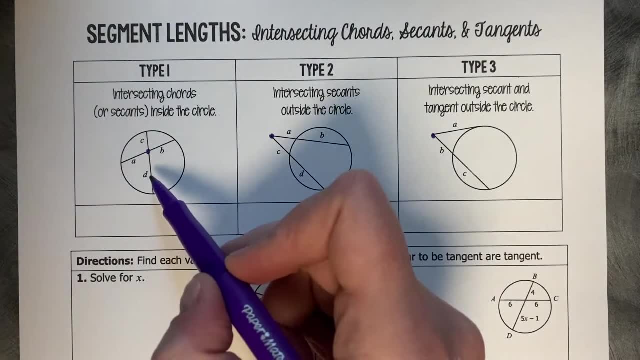 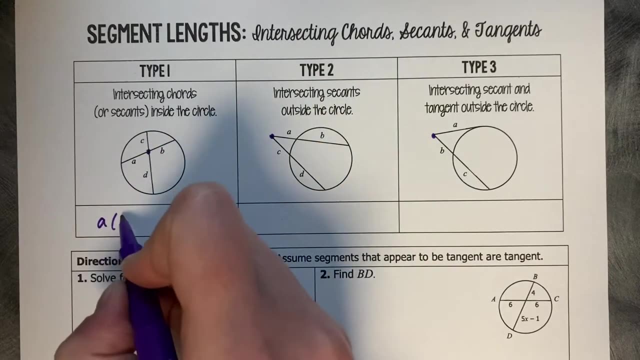 So to find any given length of these lines, they're proportionate to each other, which means you can create a proportion Well, and if you multiply it, cross multiply it, you would end up multiplying these proportionate links together. So A times B, A times B equals C times D. 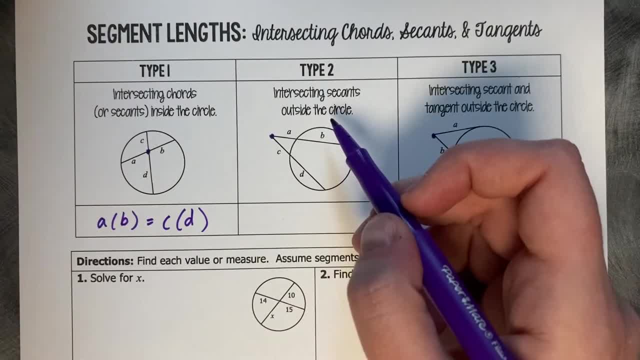 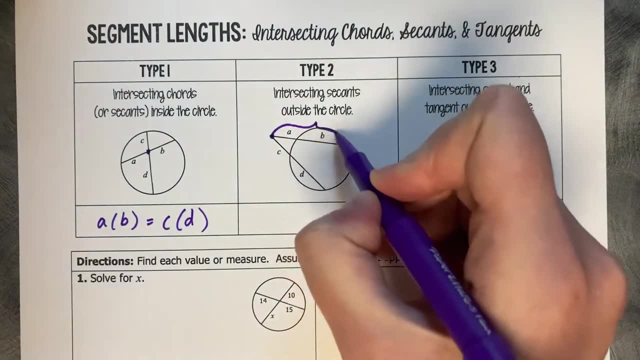 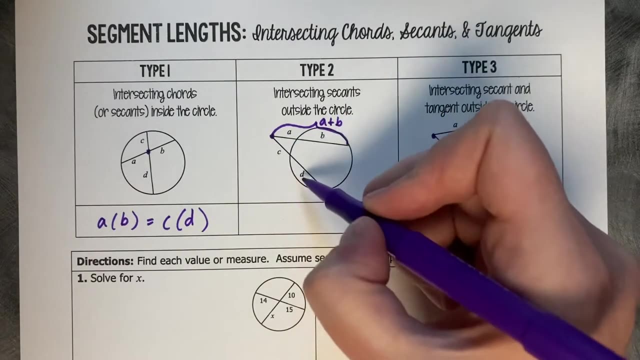 For type two. you are multiplying the segments together, but it's not just these two segments, You have to include the whole segment. So for example, this entire length here we would call that A plus B, And then this entire length we would call C plus D. 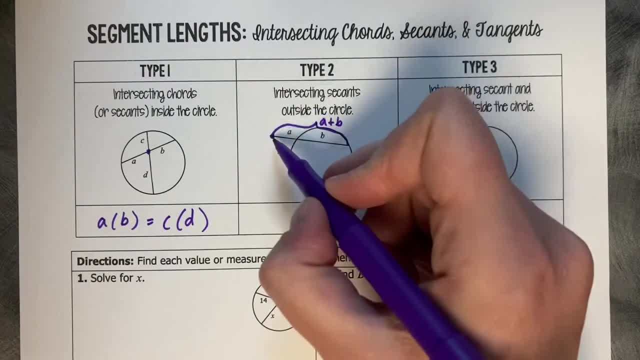 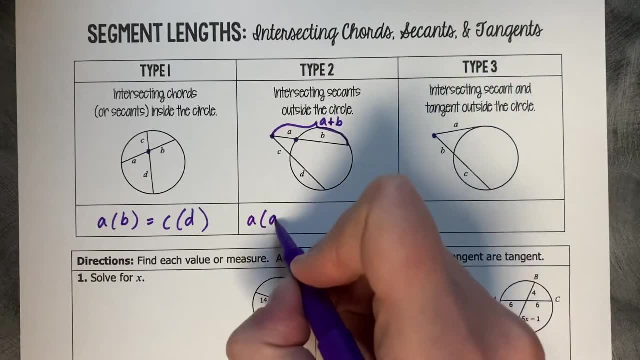 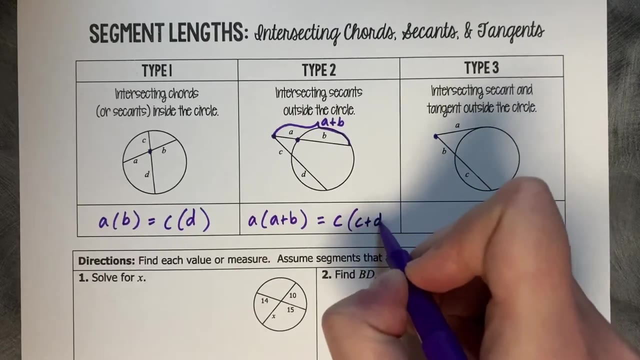 So when you multiply it, you do the length that is, from the intersection to the edge of the circle, A times the whole segment. A plus B equals the small chunk C times C plus D. So that's the whole segment. So for example, this entire length here we would call that A plus B, and then this entire length we would call C plus D. 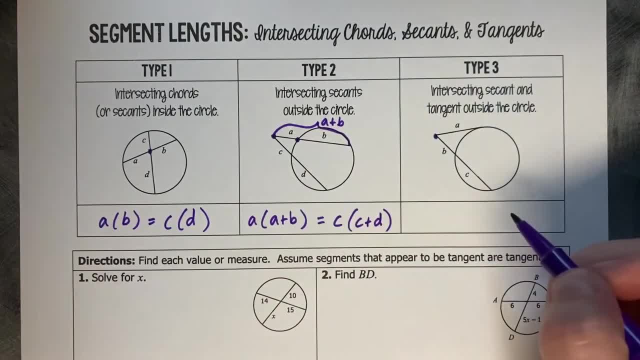 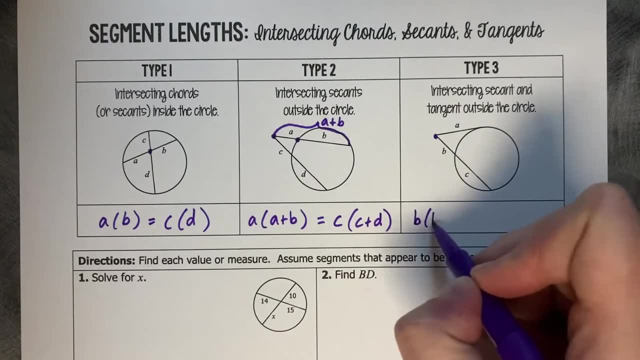 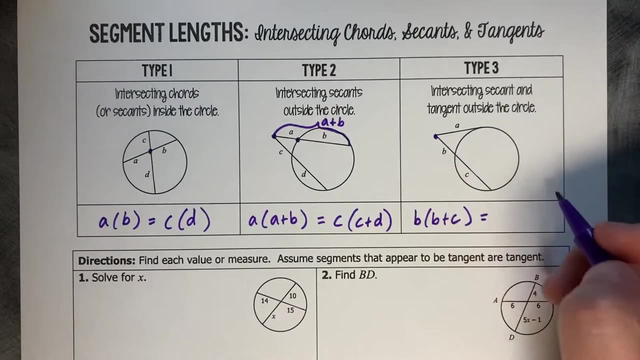 Part times whole, part times whole, And then type three. it's the same thing: B times B plus C, so part times part plus whole. And then for this one it would be part times part or part times whole, which in this case would be A times A. 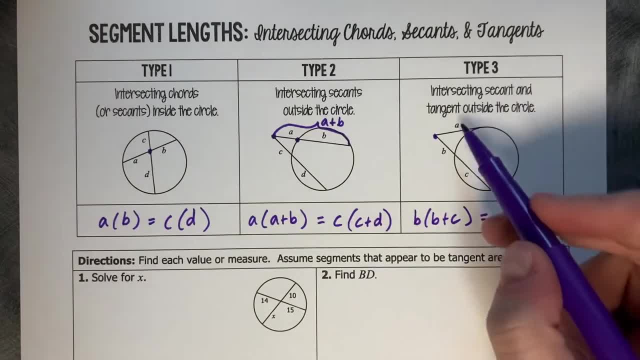 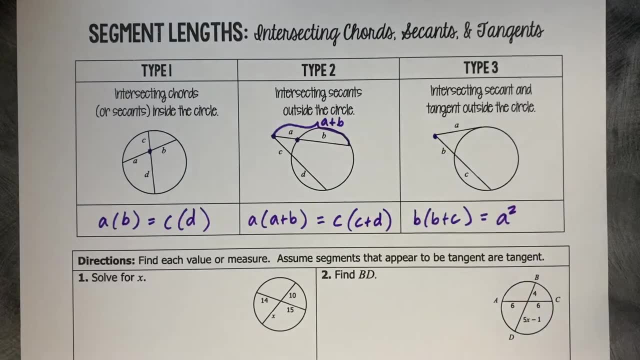 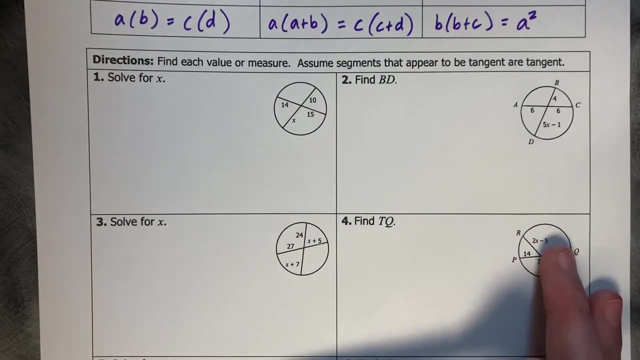 Or another way to say, that is A squared, So that little tangent is going to be squared because it's multiplying by itself. So let's try this on: Find each value or measure, assume that segments that appear to be tangent are tangent, so solve for X. 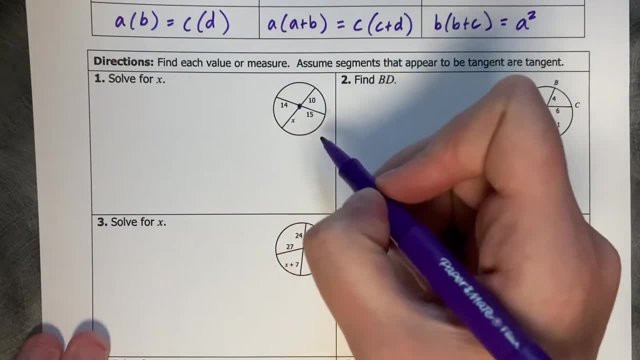 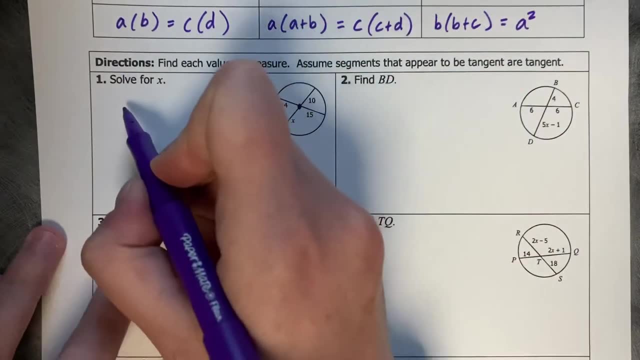 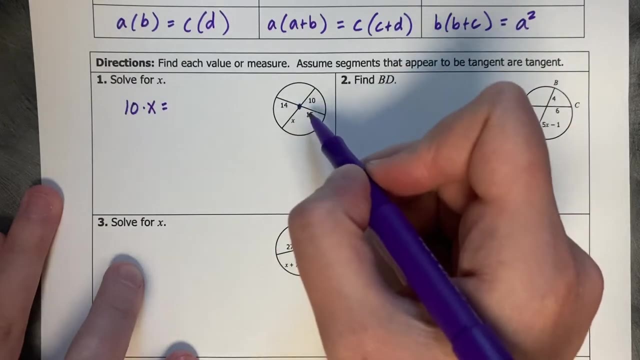 The intersection is interior, so we multiply each piece together. So X times 10, or 10 times X, whichever way you want to write it. Let's do 10 times X, And then it doesn't matter which direction you multiply this, either 14 times 15,. 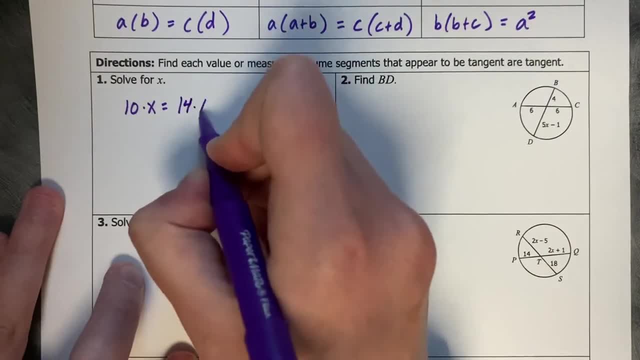 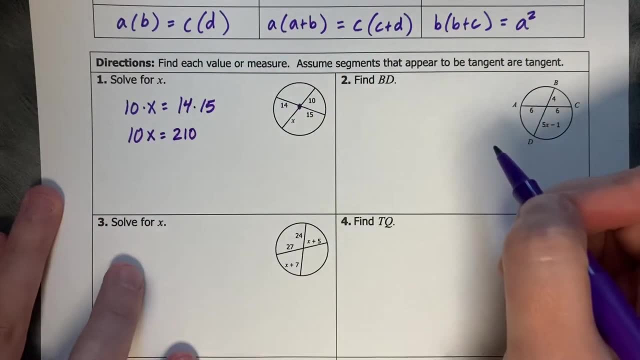 or 15 times 14,, so I'll just write it as 14 times 15.. So then this is going to be a 10X equals 210,, 14 times 15,, divide by 10, and X equals 21.. 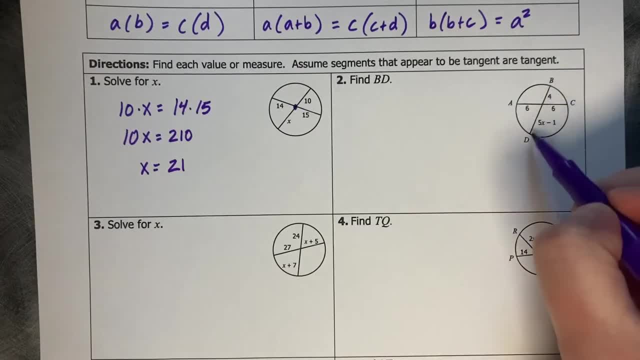 Find BD. So they eventually want to know what the whole length of this segment is here. so we're going to do a part times a part and a part times a part. so 4 times 5X minus 1.. Equals 6 times 6.. 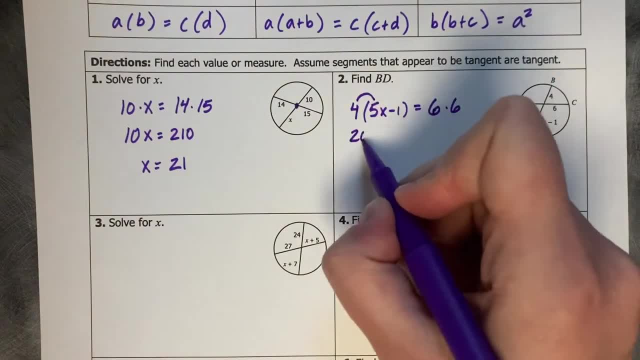 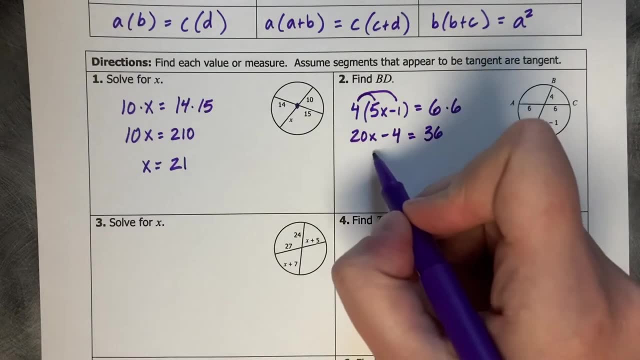 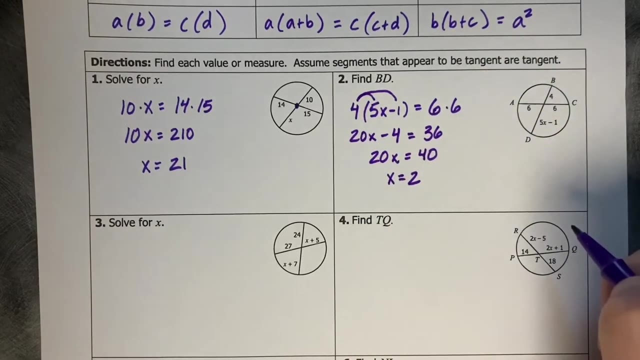 So then we distribute. so 4 times 5 is 20X. 4 times negative, 1 is negative. 4, equals 36. Plus 4. Divide by 20. So X equals 2, but we want to know the length of BD, this entire length here. 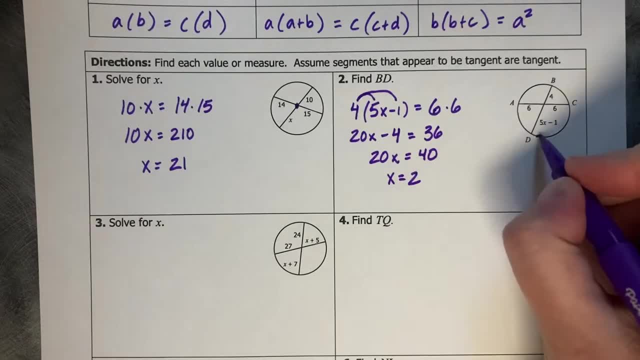 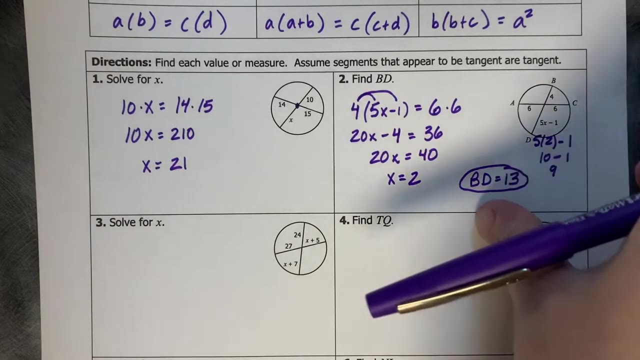 So we're going to plug it into this chunk so we can add it to 4.. So 5 times 2 minus 1.. 10 minus 1, or 9.. 9 and 4 is 13.. You try number 3, actually, no, let's do number 3 together. 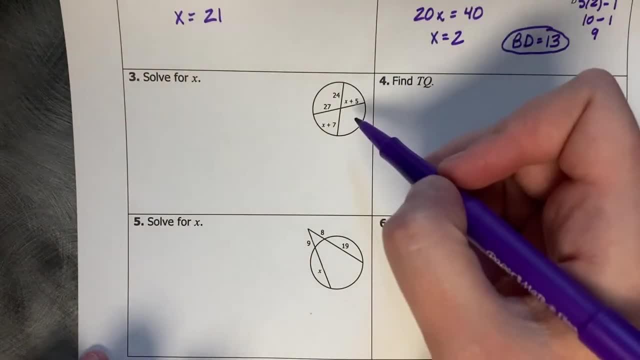 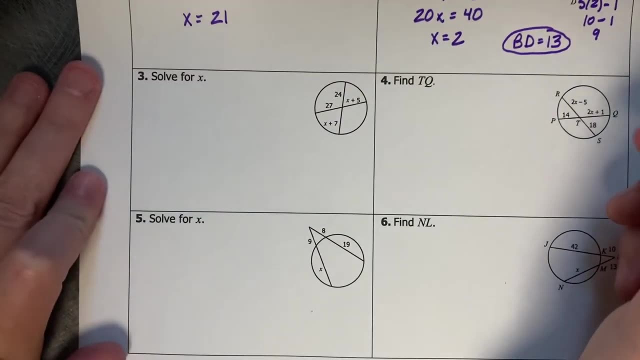 I almost said to do it on your own, but actually no, go ahead and do number 3 on your own. You can do that one, Try that one. Why didn't I do that? You can say number 3, what does that equal? 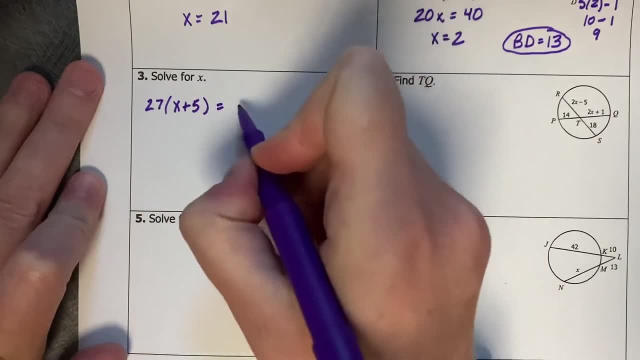 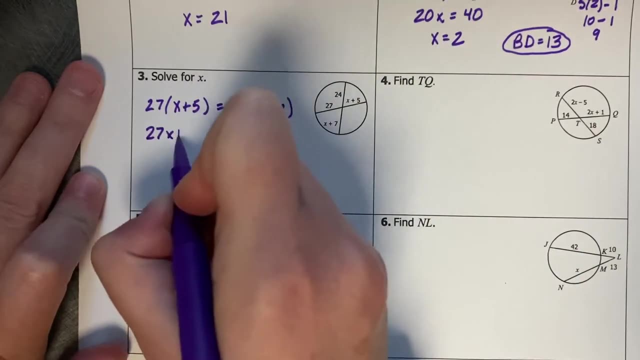 Number 3,: what does 5 half equal or 5 plus 1?? Number 3,: what does 5 half equal or 5 plus 1? 6, and what's the length of 3,, 5 plus 1?? 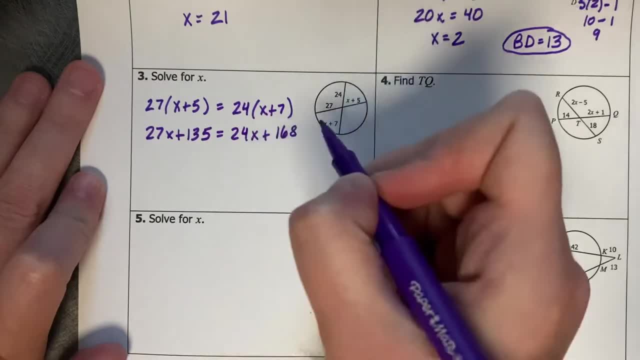 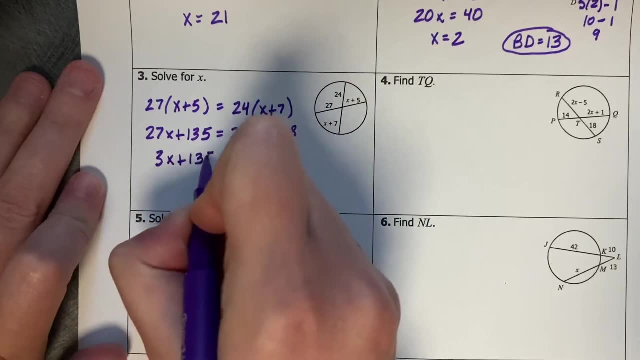 You can say number 3, what does 5,, 5, 5 equal? or 5 plus 1? 5 plus 1.. So what does 5 equal or 5 plus 1?? you can also do number four. go ahead and try that one. 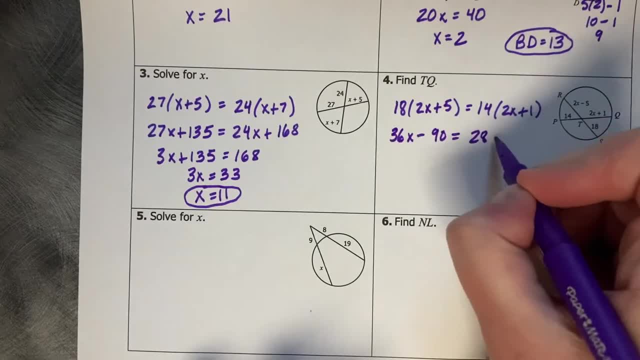 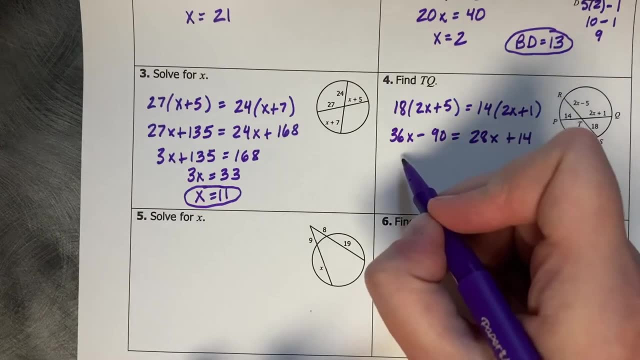 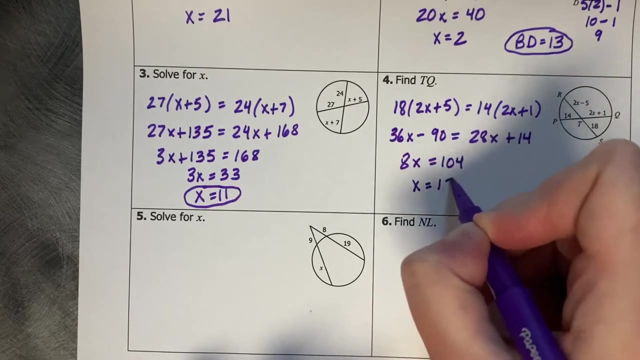 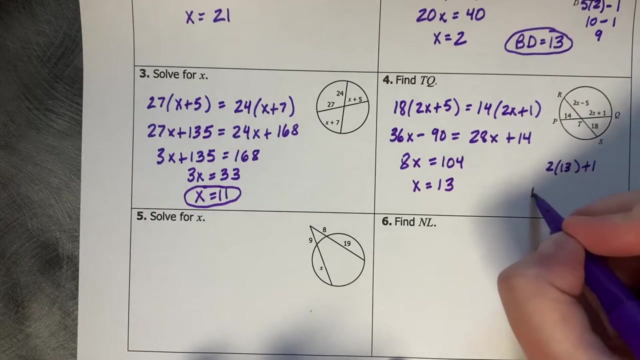 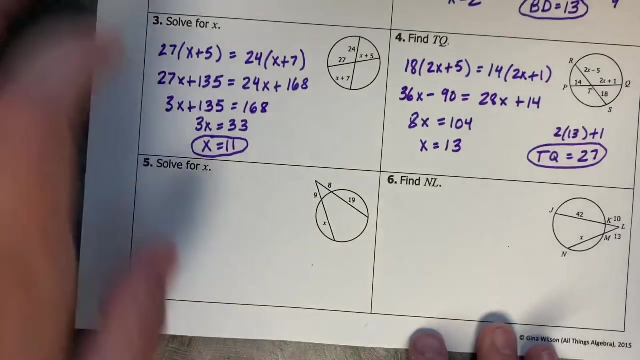 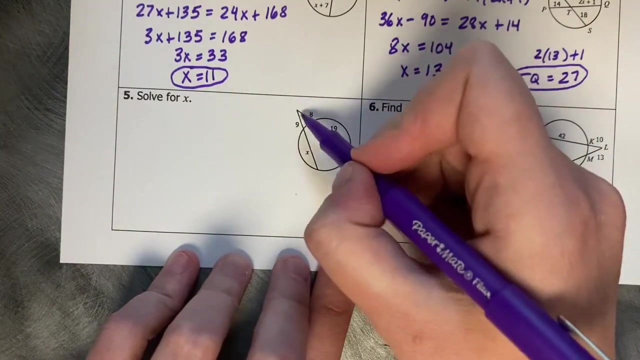 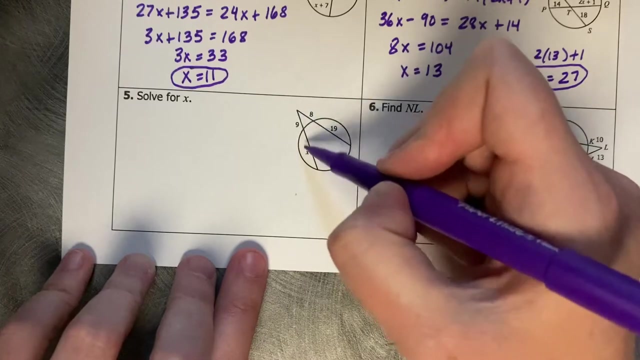 so, all right, let's try number five together. so this is an exterior point. so you're going to do your part times your whole, so you've got your 8 and your 8 plus 19, and then this guy would be a 9 times a 9 plus x. so your part times your whole and 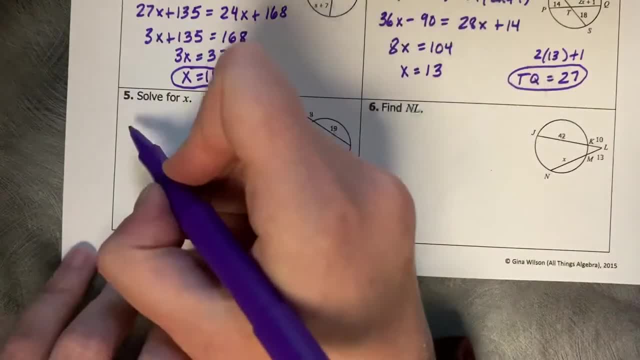 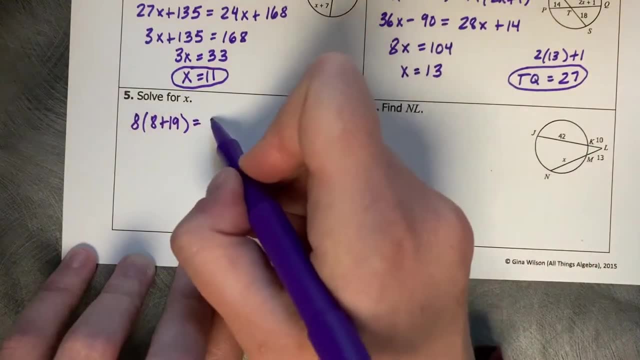 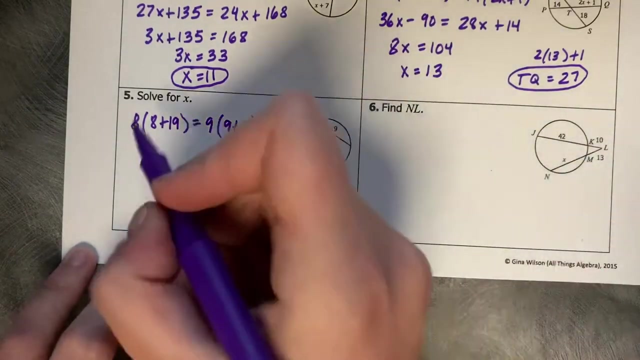 your part times your whole. so let's do this one first. so 8 times 8 plus 19 equals 9 times x plus 9, or 9 plus x. so this is going to be 8 times 27 equals, and then let's go ahead and distribute. 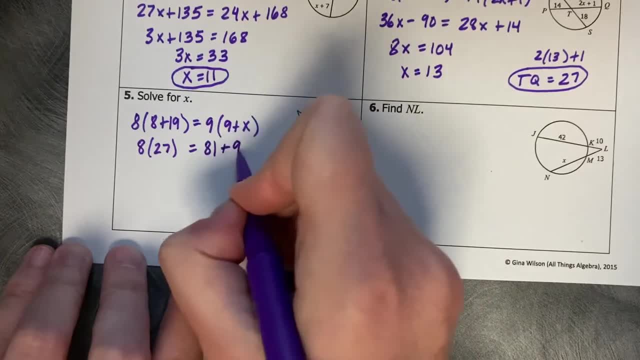 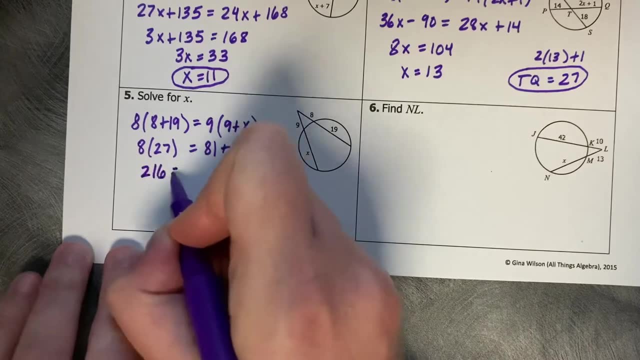 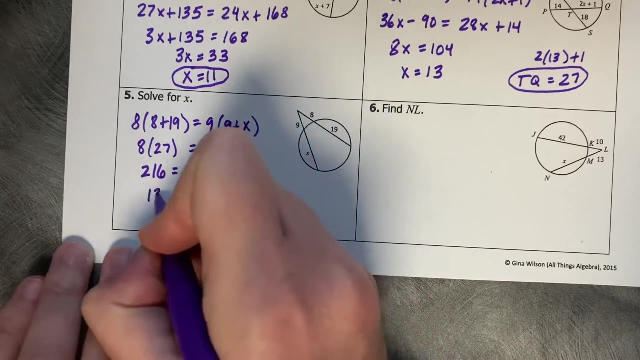 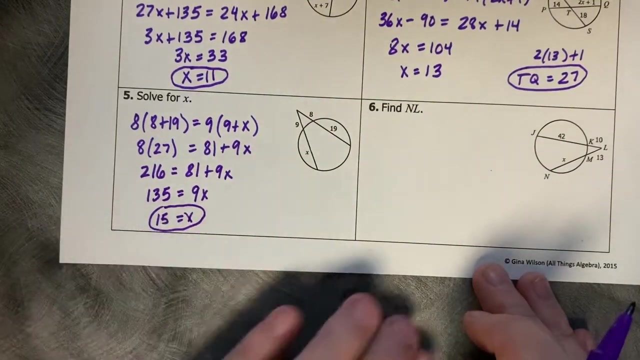 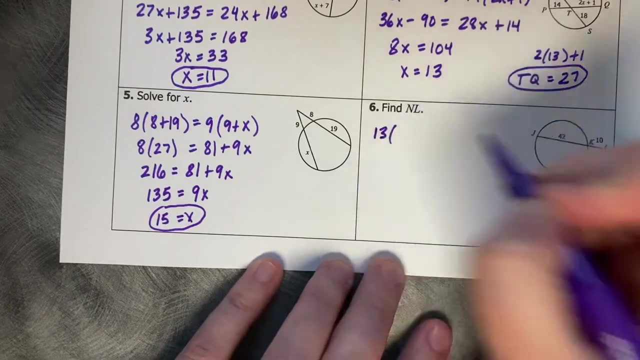 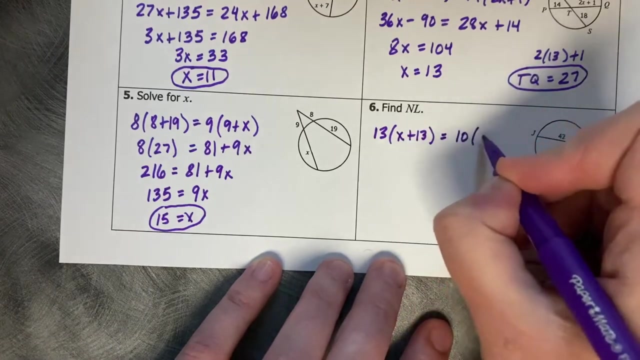 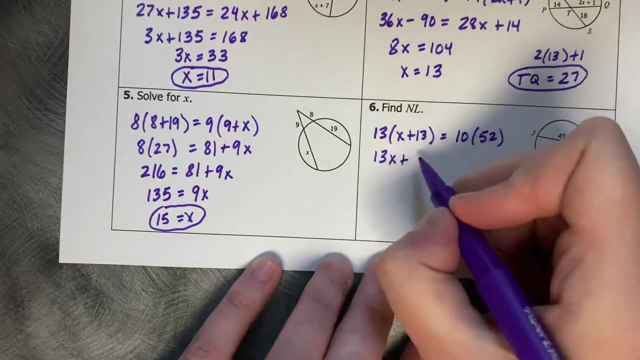 this 9 times 9 is 81. 9 times x is 9x. 8 times 27 is 216 minus 81. so x equals 15.. you try number six to get whatever you want to get right in the middle and you can wife it exactly. 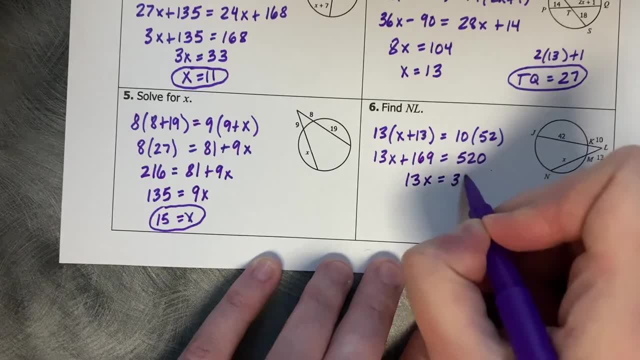 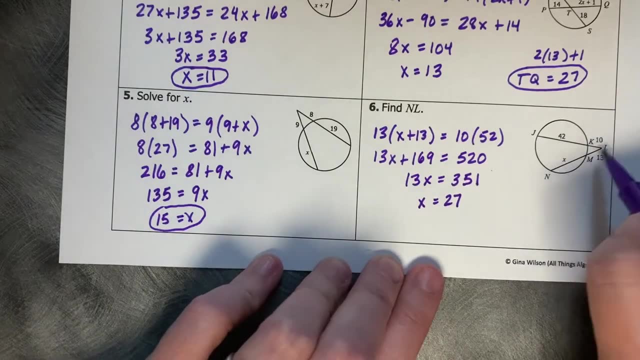 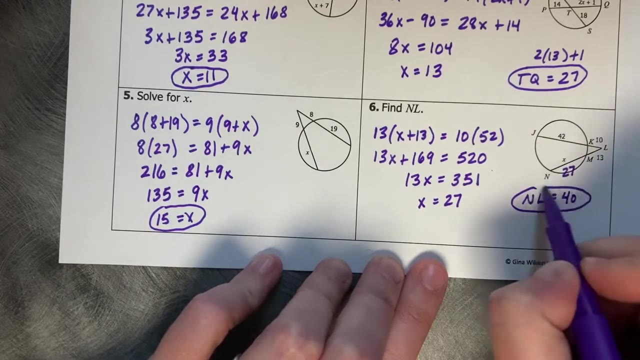 so you can eventually hide it, and we can do that if you could divide it in 4 or if you get your way. they're pretty small, but you can do that with these two Онлайн numbers, because eight times兩 n is the feet. 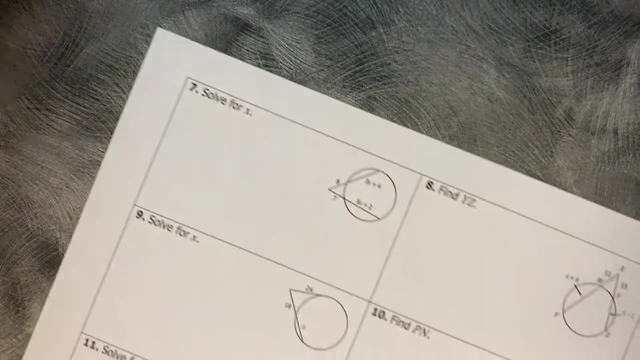 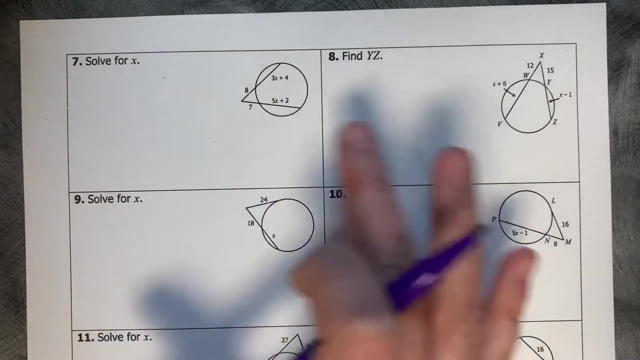 but let's name it. you're free, so that better. alltså, all right, let's get this other one. it's like 5 or 6, so 3 is one inch and that one's the biggest cup. cut yourself, guys. Seven and eight are ones you can try on your own. 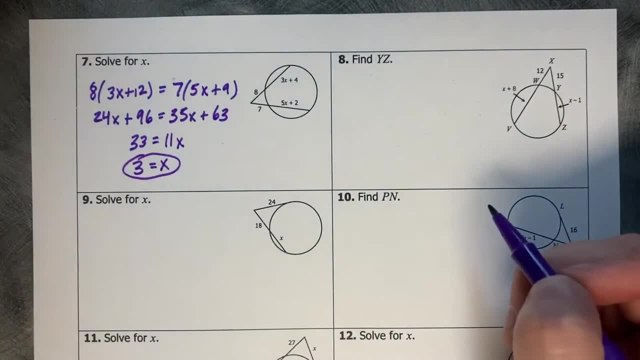 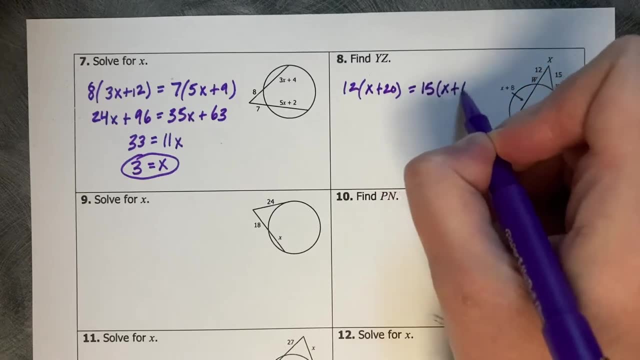 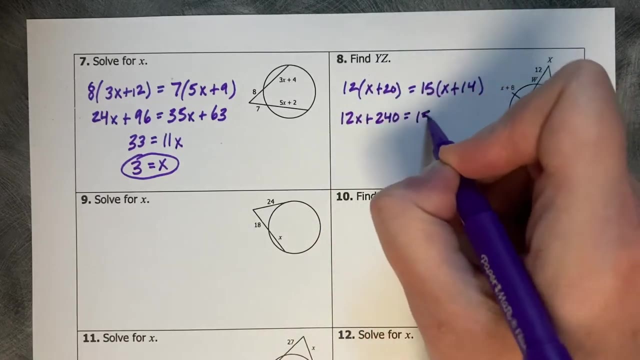 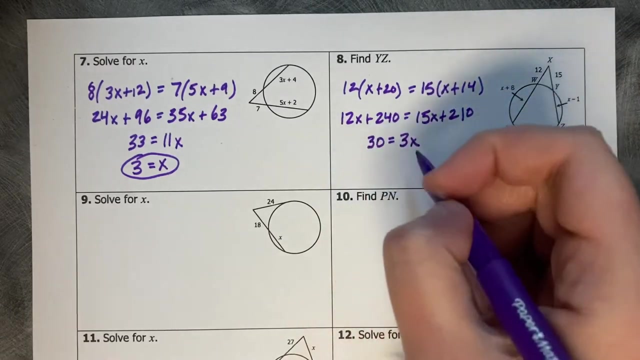 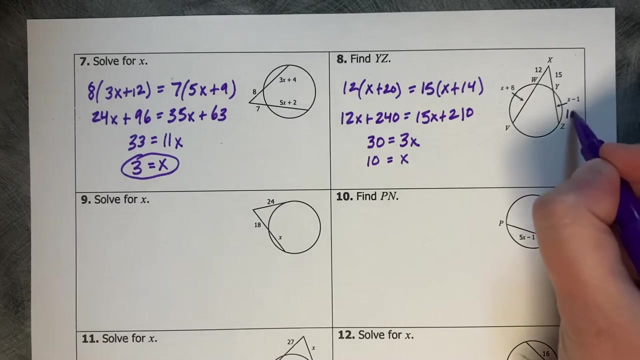 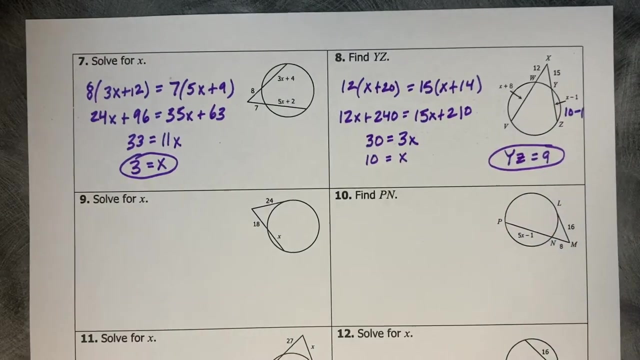 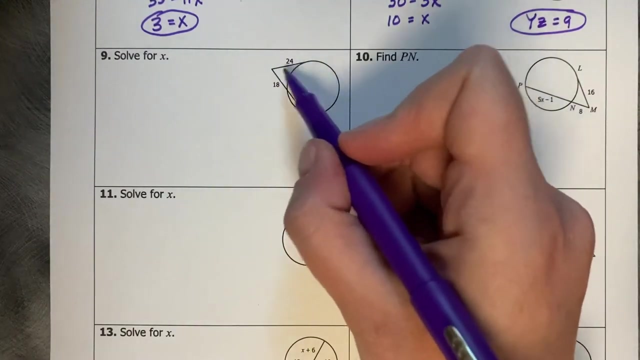 All right, All right, Let's take a look at number nine together. The difference between this one and the last couple is that I have one secant and one tangent, So that length of 24 does not go inside of the circle, but you use it. 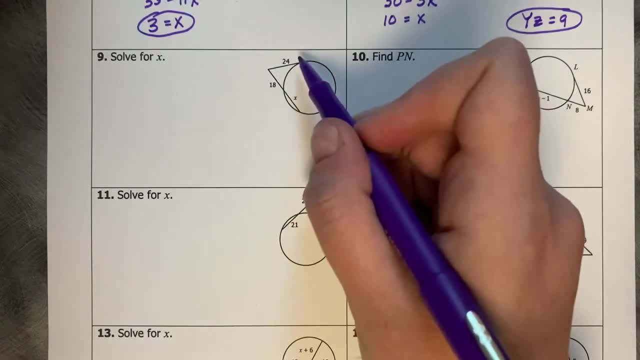 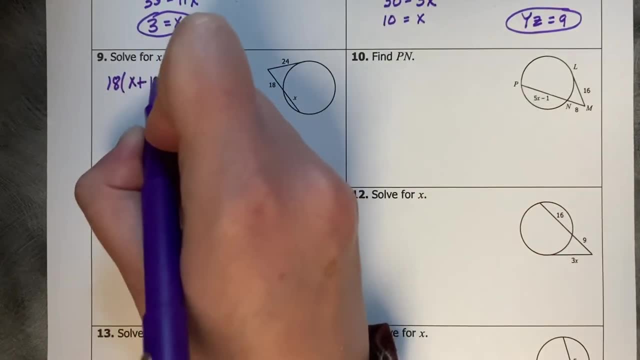 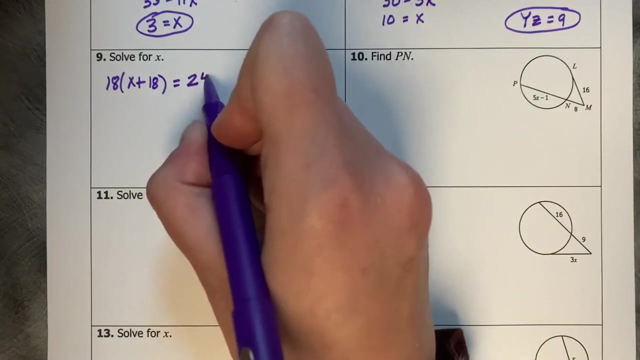 You're still doing a. you know part times a whole, but the part and the whole of the same number. So let's do this piece first, So 18 times X plus 18.. Part times the whole And then part times the whole. on this one is 24 times 24, which is going to be 24 squared. 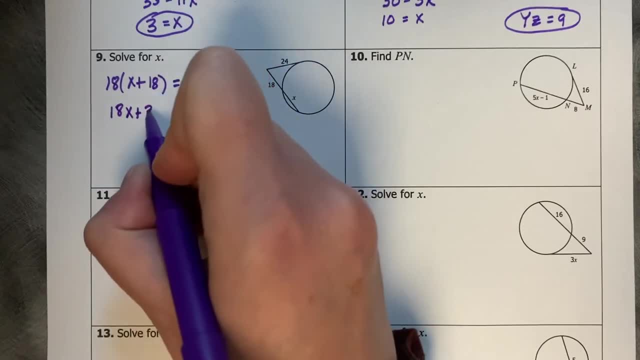 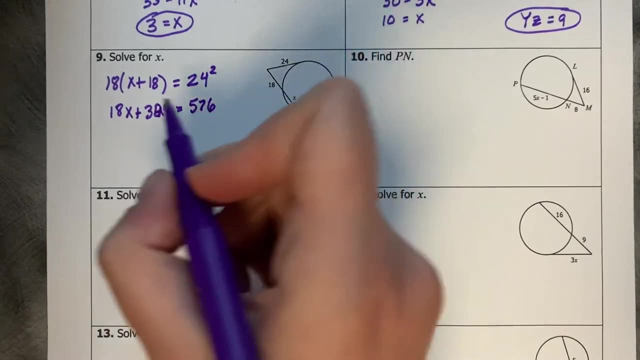 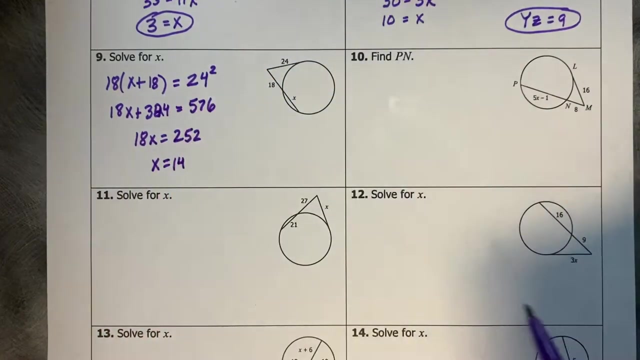 So then we've got 18X plus 324.. Whoops, 24.. And then 24 squared is 576 minus 324, 252, and X equals 14. So that's six times the whole Similar one here. 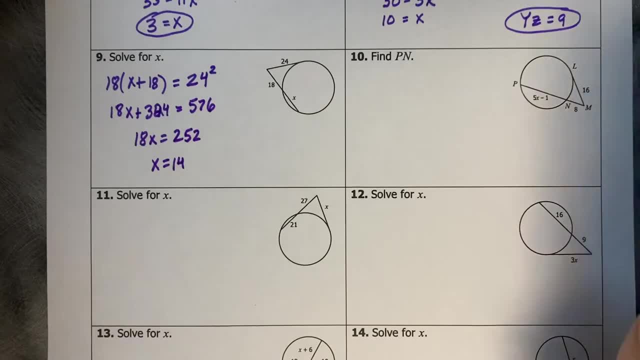 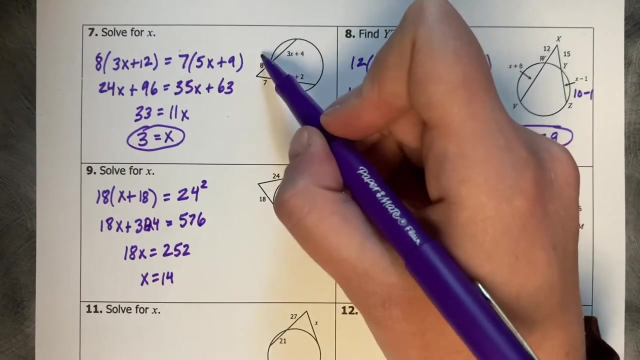 Go ahead and try this one. Oh, I missed kind of showing something up here. So part times the whole on this one. the whole, you do the eight and the four together. I just wrote it but I didn't actually explain it. 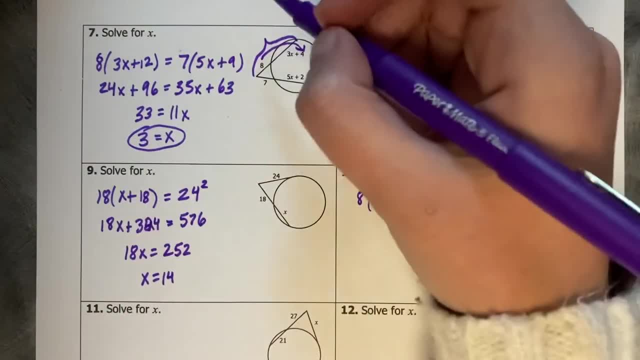 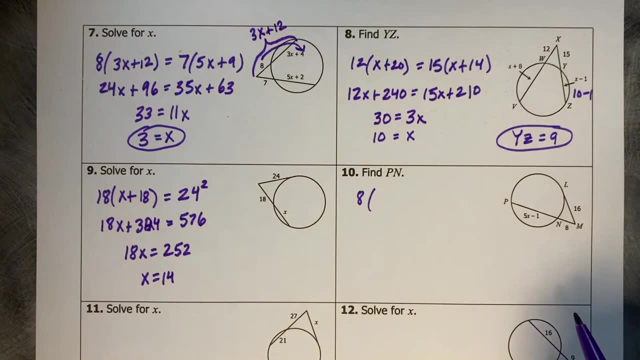 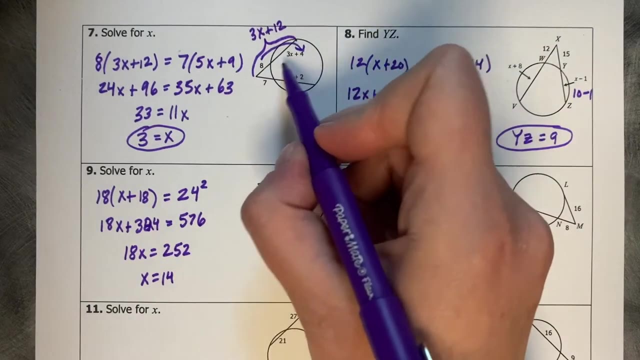 So this is where the 3X plus 12 came from. So that's going to be a 3X, eight and four to make 12.. I'm sorry, I did not highlight that, It's just moving too quickly. So don't forget that when you add those together, those constants, the eight and the four, or 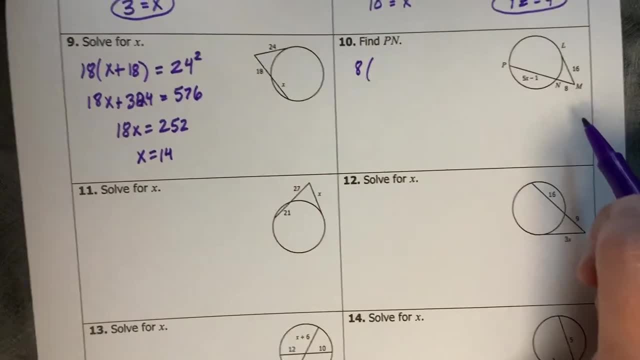 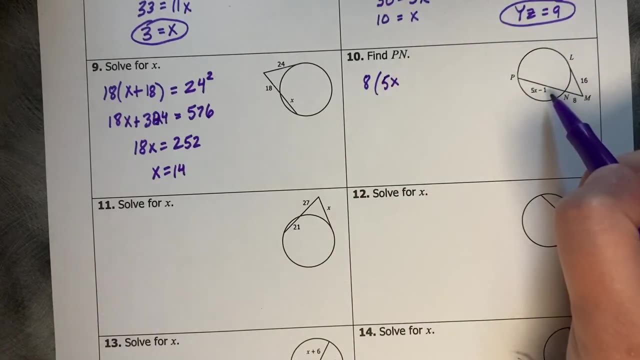 the seven and the two would go together for the whole. So let's try this one. So this one's going to be an eight times a 5X, And then the eight minus one is going to make that a seven. Seven Equals 16 squared. 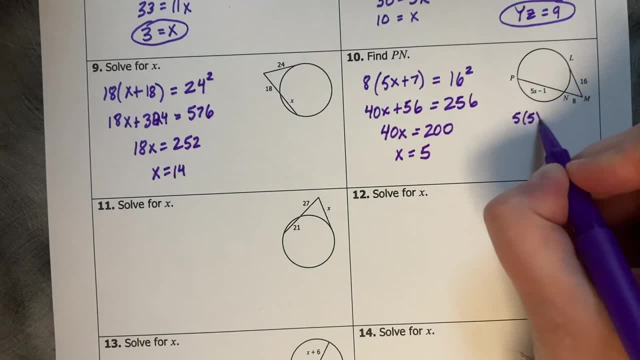 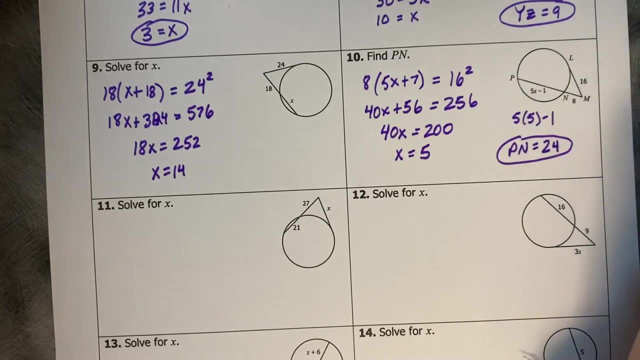 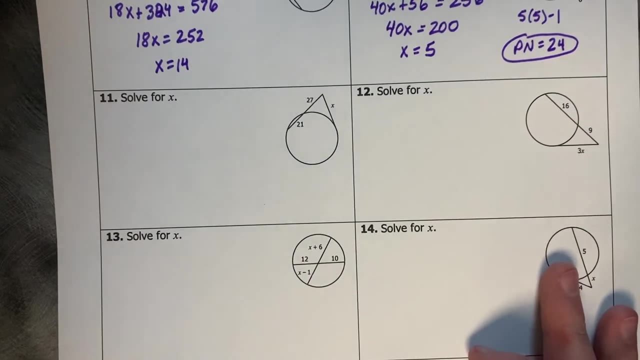 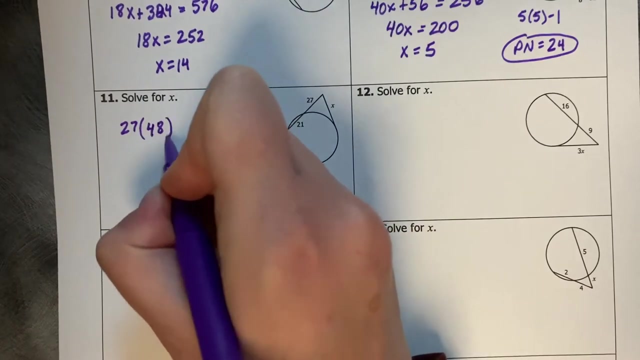 And then plug it back in for PN 25 minus one, 24.. All right, Let's take a look at this one. So part times a whole, 27 times 27 plus 21,, which is 48.. And then a part times a whole. on this one is an X and an X. 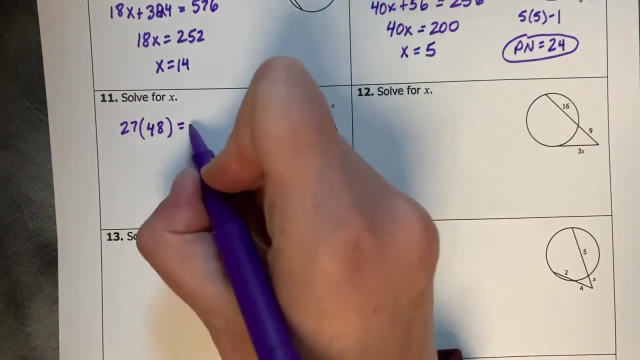 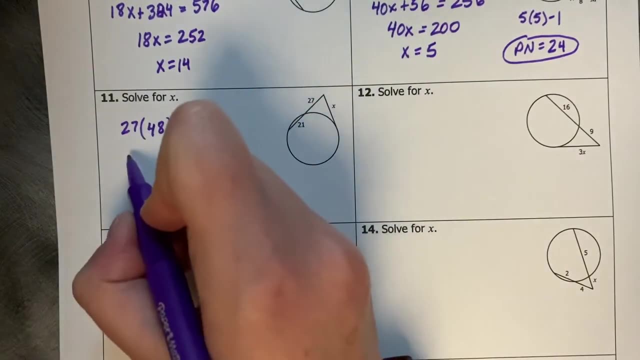 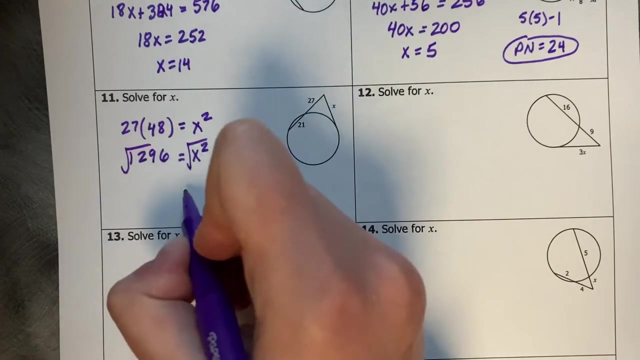 And an X times an X is not a 2X, It's an X squared. So then we've got: X squared equals 1,296, and the opposite of a square is a square root, And the square root of 1,296 is 36.. 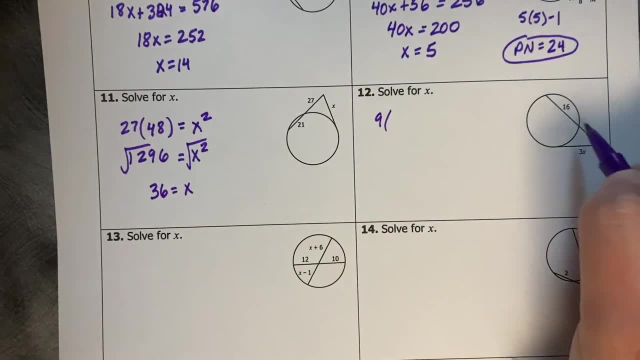 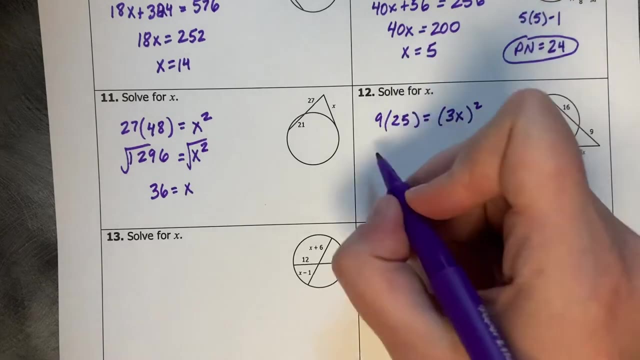 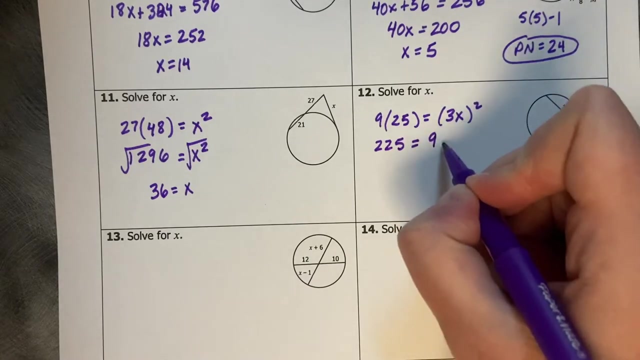 Let's try this: one Nine times nine plus 16, which is 25, equals part times part or whole times whole. So 3X times 3X, squared Nine times 25, is 225.. 3X times 3X is three times three, which is nine, and X times X, which is X squared. 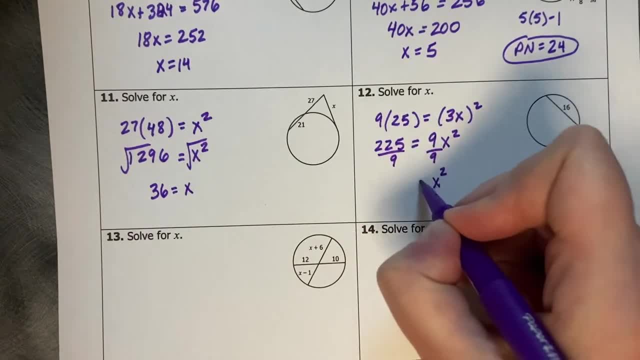 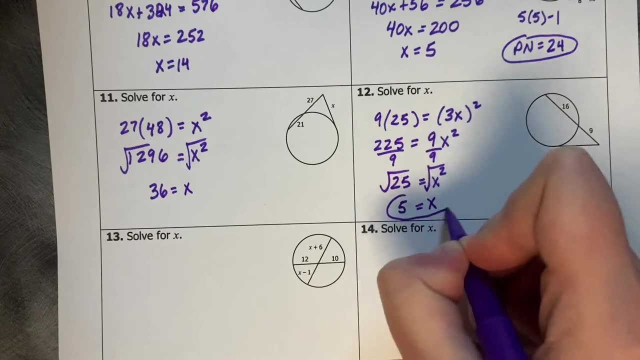 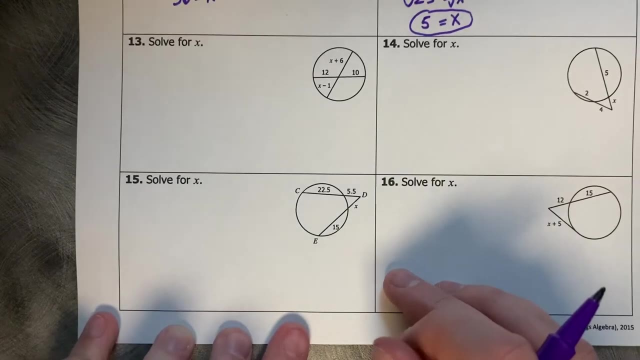 Then we divide both sides by nine, So we get X squared equals 25.. And the square root of 25 is five. Okay, So that's root of 25.. All right, We're back to an intersection in the middle here. 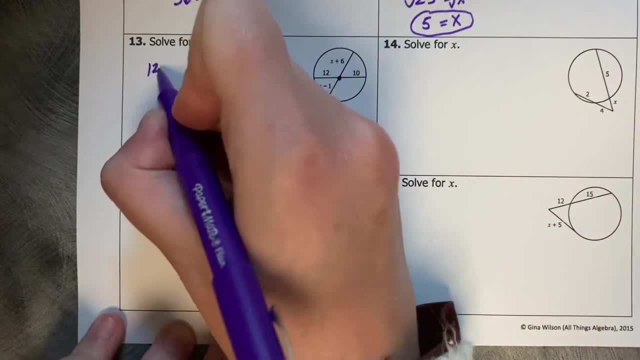 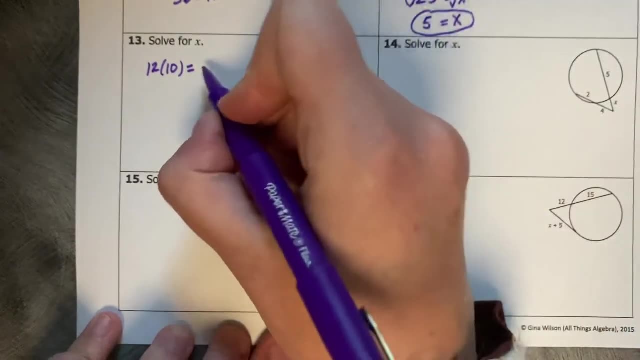 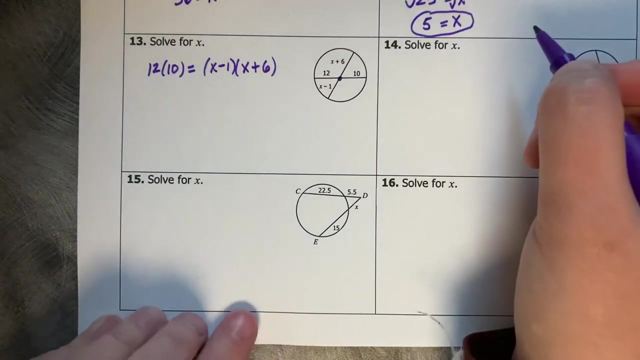 So you've got to multiply each piece together, So 12 times 10, and then these two pieces both have X's. Make sure you group them together with parentheses. So X minus one times X plus six, 12 times 10 is 120. 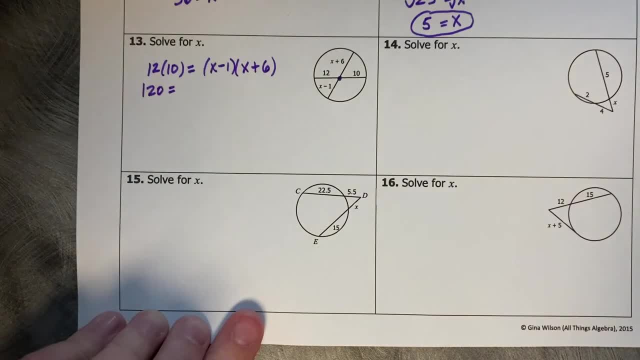 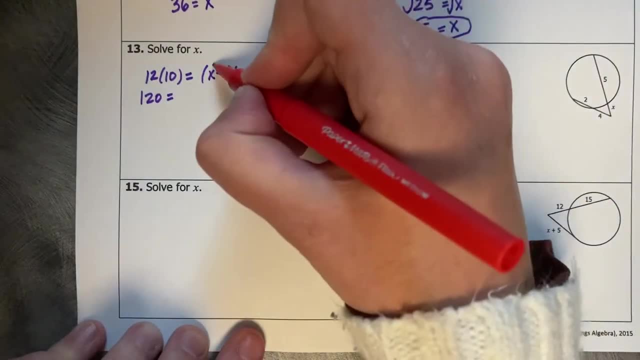 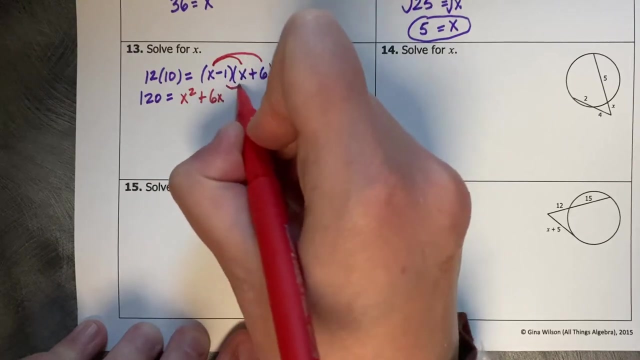 And then, on this right hand side, we're going to double distribute, or double distribution, or what you might have learned as FOIL: first outer, inner, last. So x times x is x squared, x times 6 is 6x negative, 1x negative, 6.. 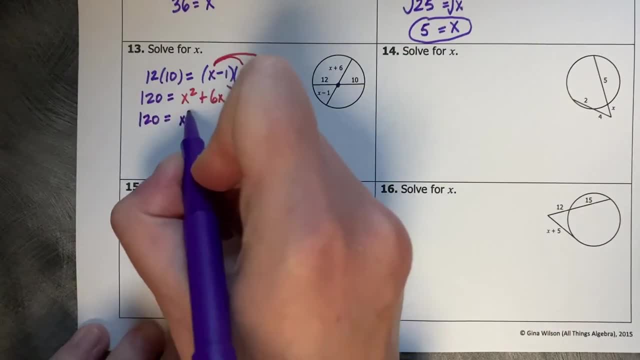 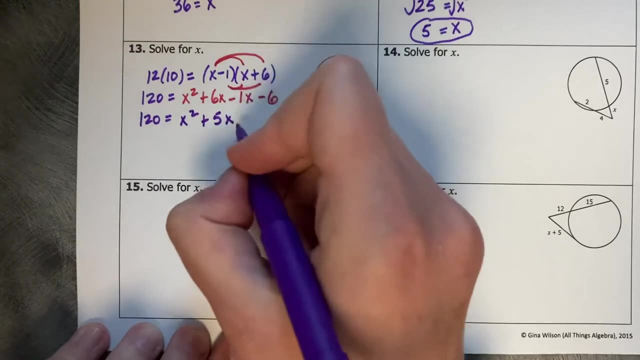 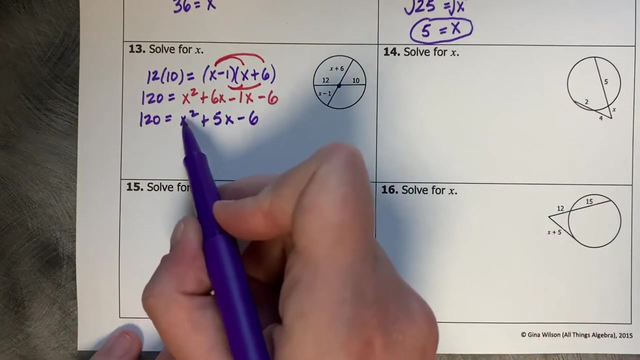 So then we've got 120 equals x squared, And then 6x minus 1 is 5x minus 6.. And now this equation is a quadratic. I can see it's a quadratic because it's got an x squared and it's in a trinomial form. 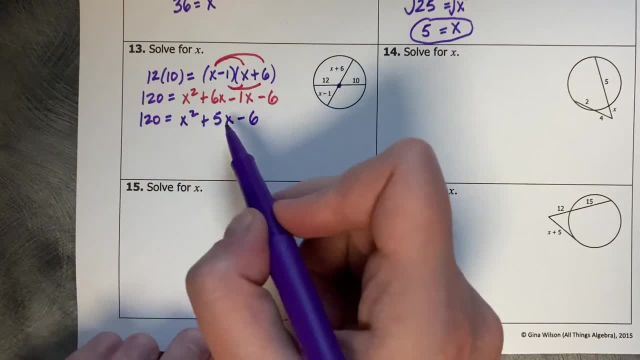 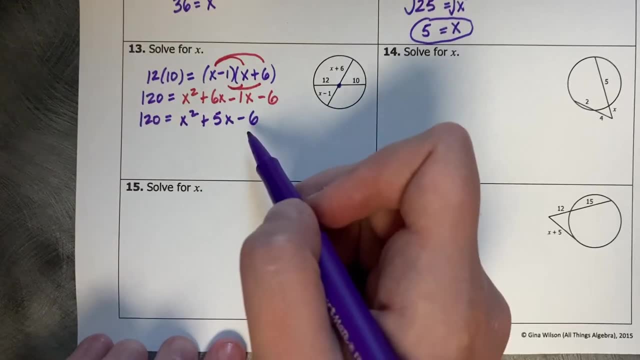 x squared 5x minus 6, where it's a ax squared plus a, bx plus a c, And so if we want to solve this very efficiently, the best way to do it is to factor, And factor may look different for different people. 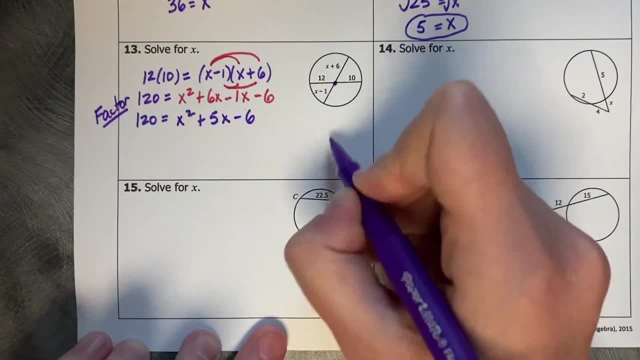 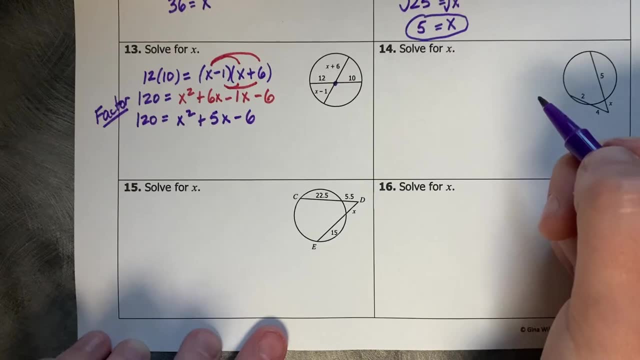 Some people like to use the area model, the box where you put it in the four squares, Or some people use grouping, which is still the very first thing you need to do is get your equation equal to 0.. So the first thing you do is subtract 120.. 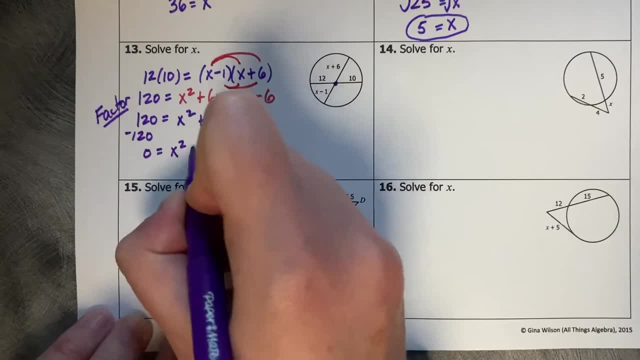 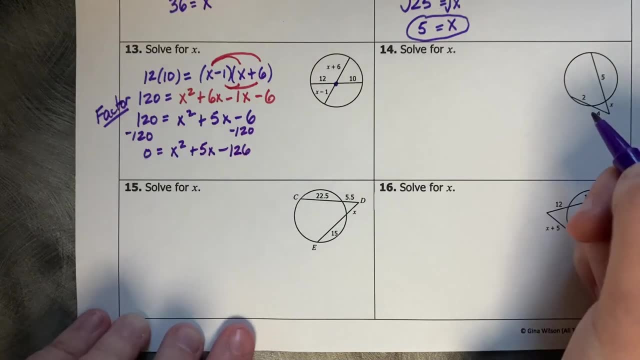 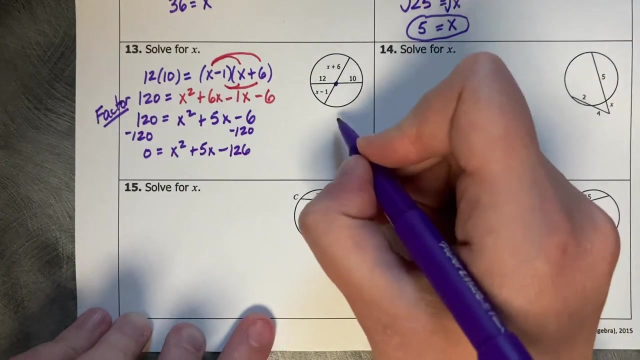 So then we get 0 equals x squared plus 5x, And then now it's minus 126.. And then you do a times c, In this case an a is a, 1. So 1 times negative 126 is negative 126.. 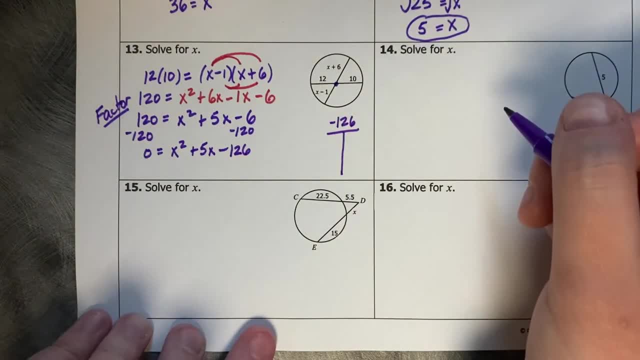 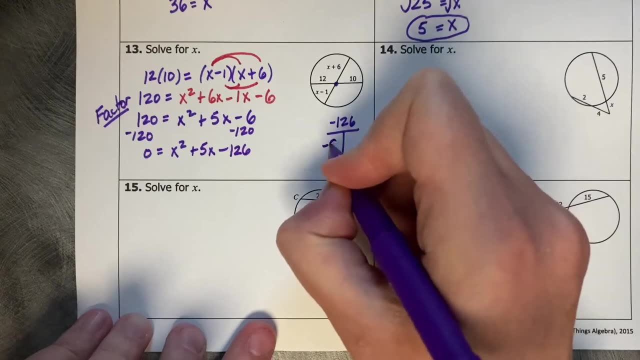 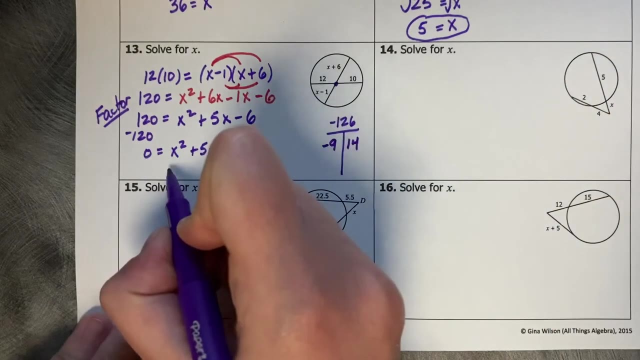 And then I like to draw a little t-table to give me my factors of 126.. And I just know this one off the top of my head: that 14, a negative 9 and a 14 multiply to negative 126. So then our factors are x minus 126.. 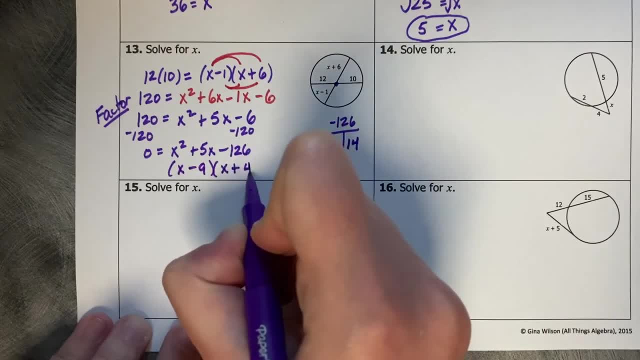 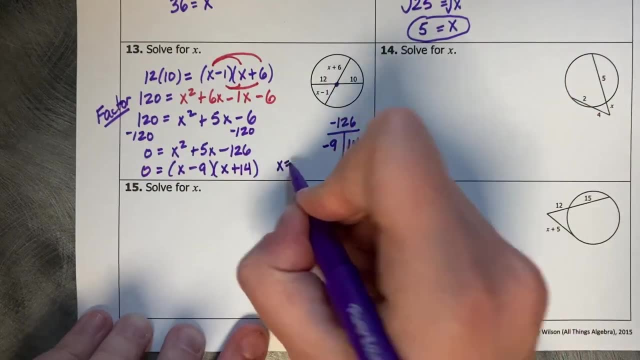 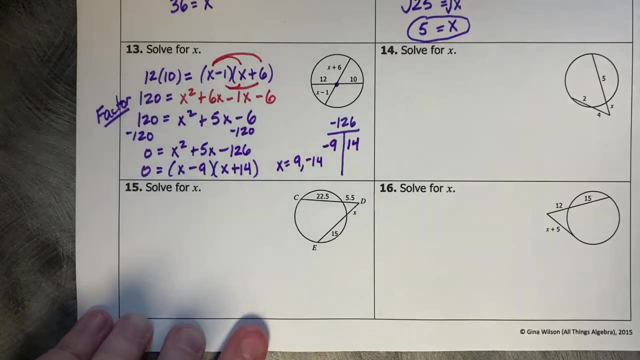 9 times x plus 14.. And then equals 0.. So then our two solutions are: x equals 9 and x equals negative 14.. Well, in this case, negative 14 cannot be a solution, as we're not working with negative values. 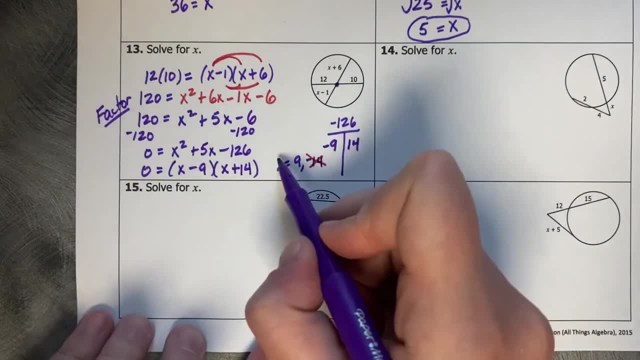 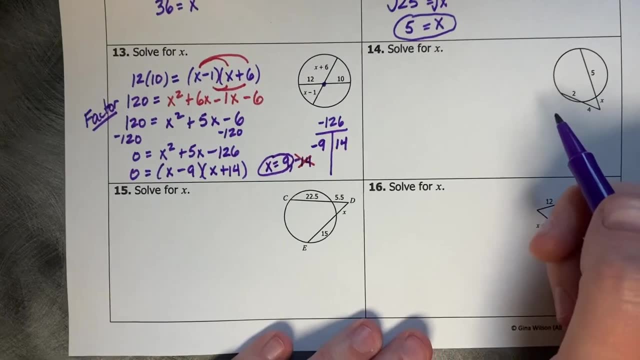 So if I had negative 14 plus 6, this would be a negative length. So the only true solution in this case is x equals 9.. On the next one I'll show the area model X times, or do the part times the whole, part times the whole. 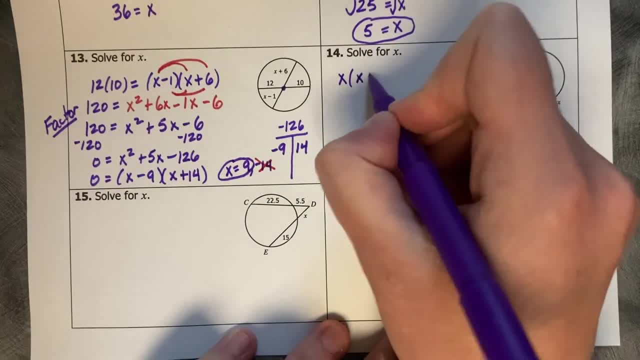 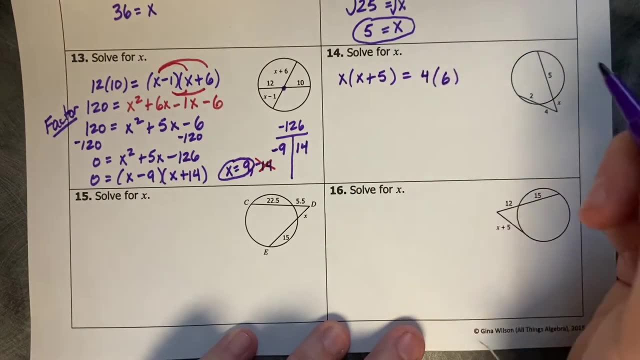 So we got x times x plus 5.. 4 times 2 plus 4 or 6.. x times x is x squared, x times 5 is 5x, equals 24.. Again, I've got a quadratic x squared and a 5x. 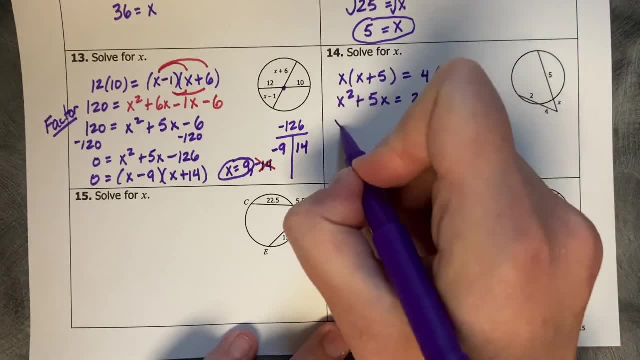 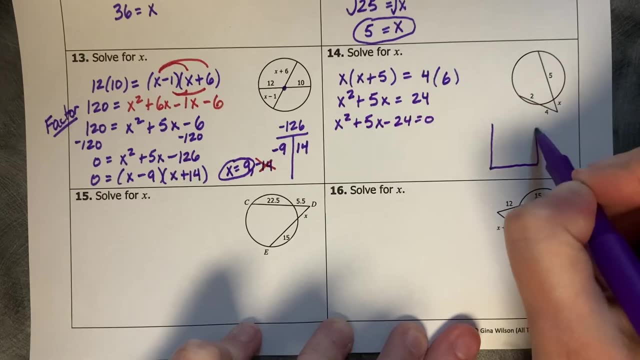 I've got a constant, so it needs to be equal to 0.. So subtract 24.. And now I'll show the area model. So you put your x squared in this box And the negative 24 down here, And we want our 5x to be split evenly between these two boxes. 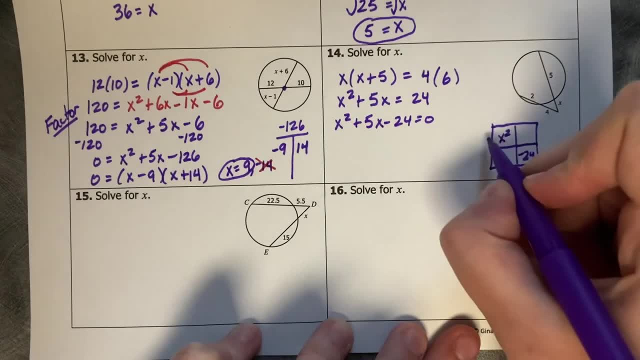 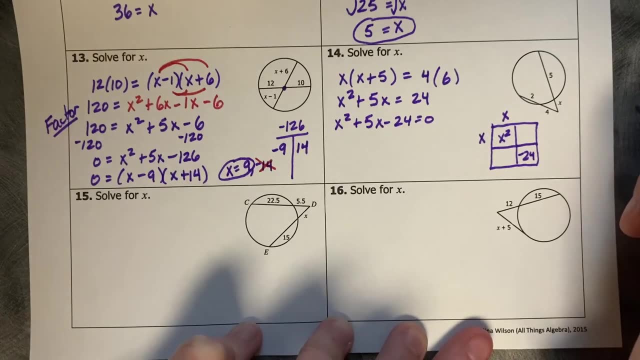 But how do we split them? Well, we have to work backwards. So we know we've got an x and an x And you have to say what two numbers multiply to negative 24 but add to 5. So we've got negative 24.. 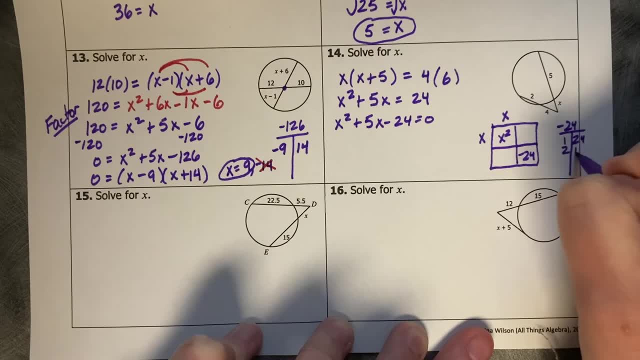 And you can do the whole table. So 1 and 24,, 2 and 12,, 3 and 8. And I think those are the pairs, But you could go one more: 4 and 6. So it's definitely 3 and 8.. 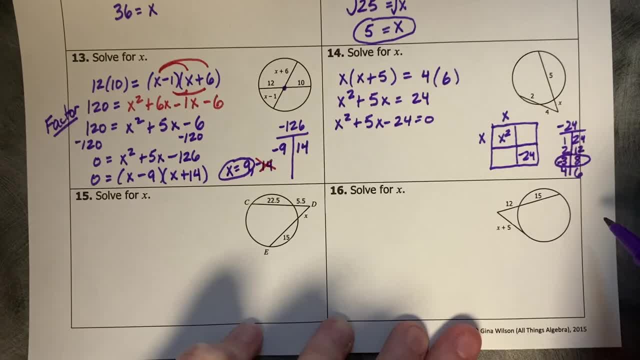 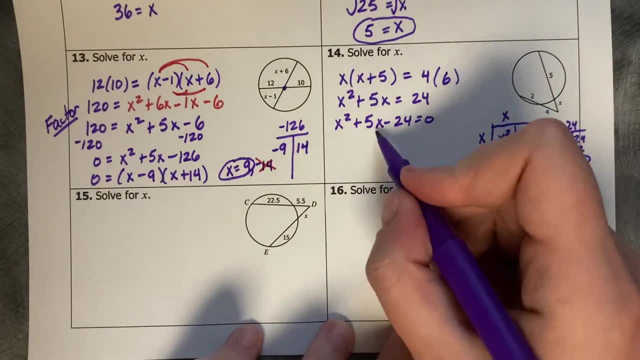 And the 3 is negative because I want it to be a positive 5.. So it's going to be a negative 3x and an 8x, because 8 minus 3 is 5.. So then this is an 8 and this is a negative 3.. 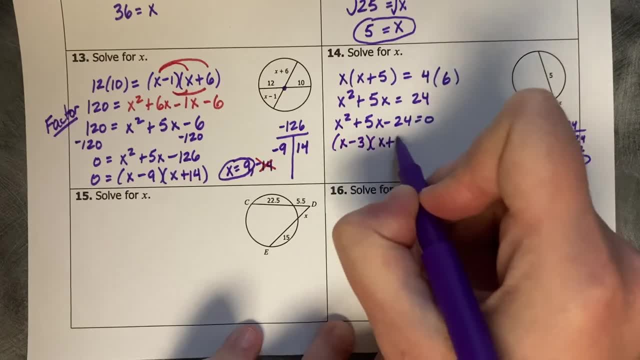 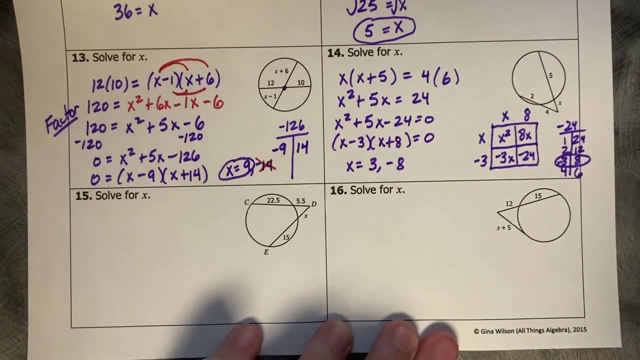 So then our factors are x minus 3, x plus 8 equals 0. So our two solutions are 3 and negative 8. But again, negative 8 can't be a solution here, because we're only looking for positive values.